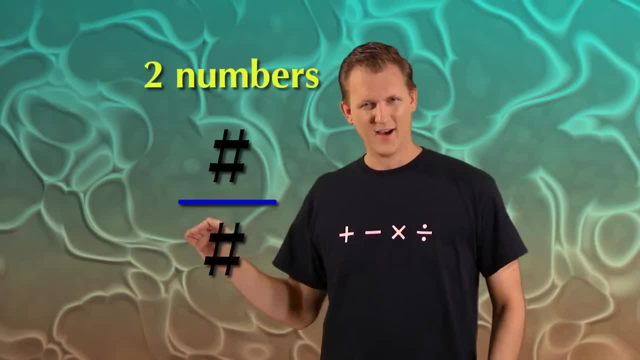 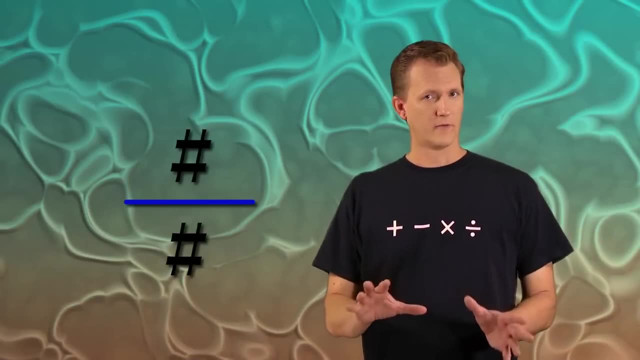 One number on top, one number on bottom and a line between them. I'll explain exactly what the line's for later in the video, But for now let's figure out what those two numbers mean. Remember, fractions are used to represent parts of something. 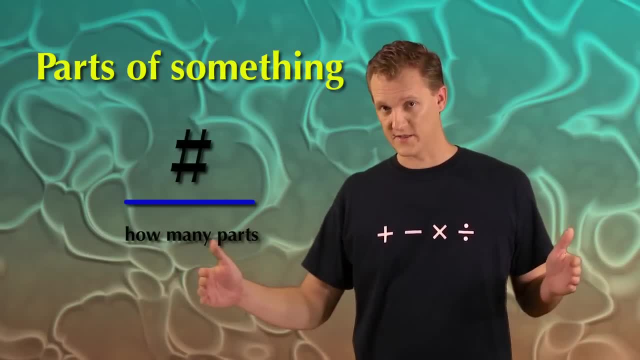 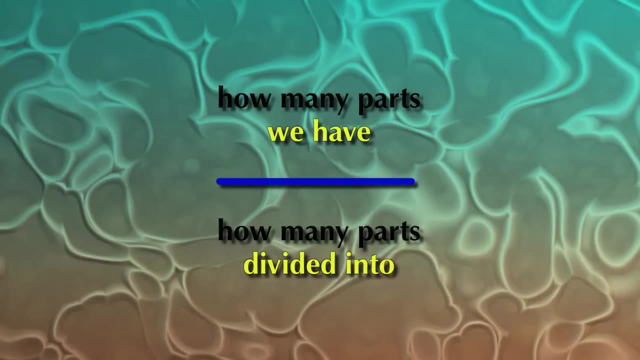 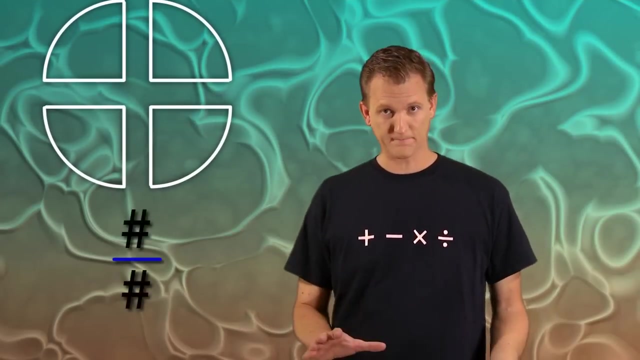 And the number on the bottom tells us how many parts that something is divided into. The number on top tells us how many of those parts we have. For example, let's write a fraction for our drawing here. I divided the circle into four parts, right? 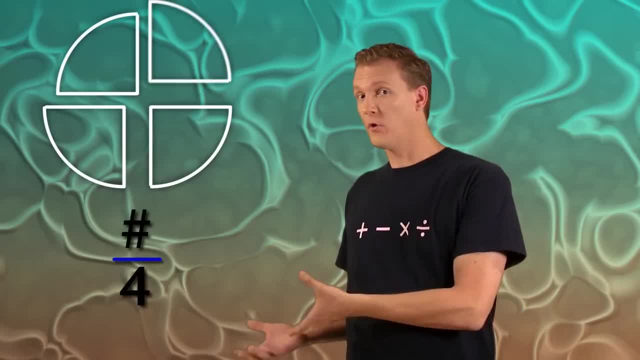 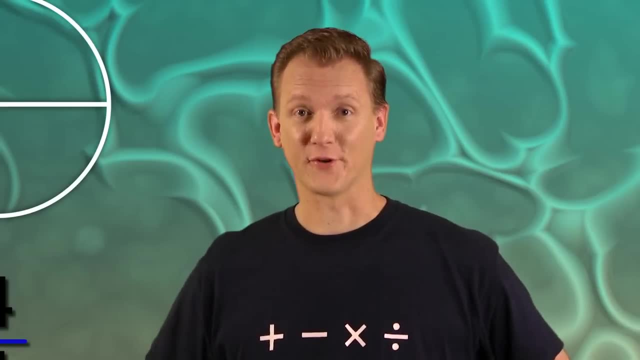 So the number on the bottom will be four. And I still have all four of those parts. so the number on top will also be four. I have four out of four parts. That means I still have a whole circle. But what if somebody came by and took away one part from the circle? 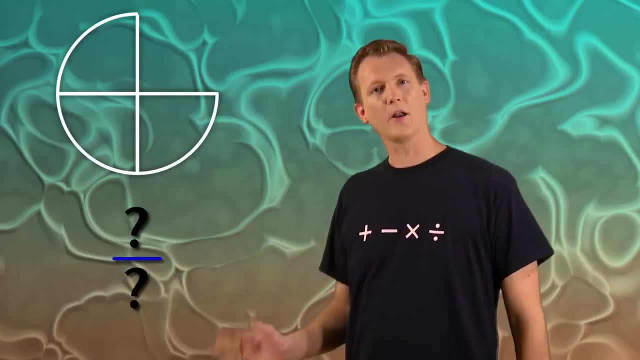 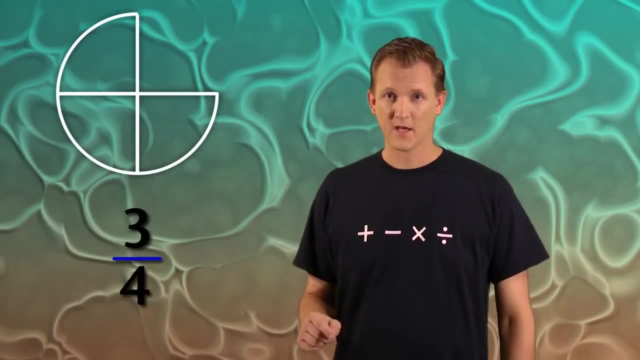 Well, the circle's still divided into four parts, so the bottom number would still be four. But I only have three of those parts left, So that means the top number will change to three. So I have three over four or three-fourths of a circle. 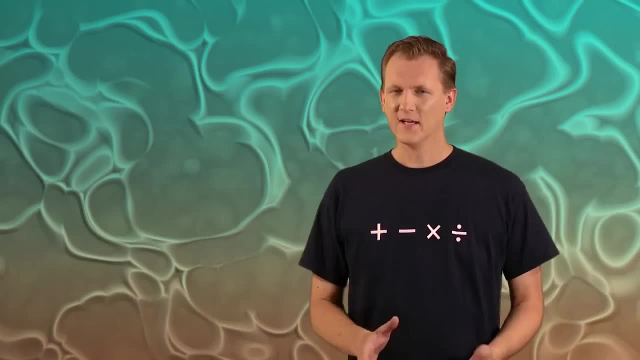 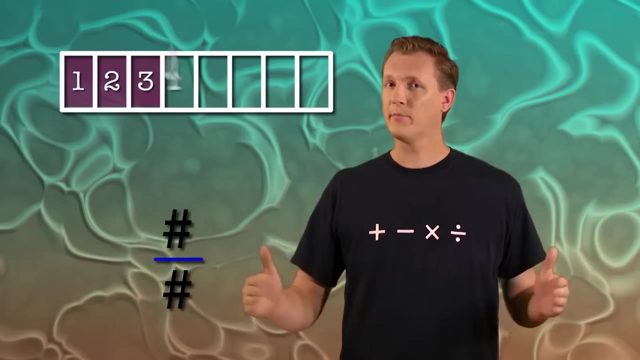 Make sense. so far Good. Let's try another example. Let's say that I divide a rectangle up into eight parts And I give you three of those parts. Since the total number of parts is eight, the bottom number will be eight. 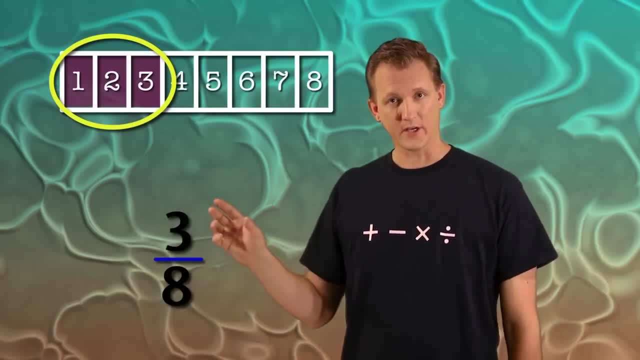 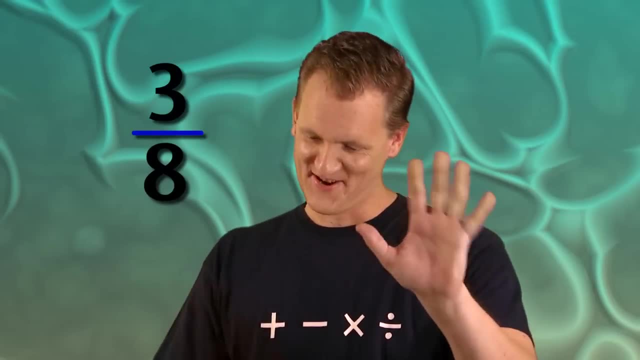 And since you have three of those parts, the top number will be three. So the fraction I'm giving you is four. That means three over eight or three-eighths of the rectangle. No, no, no, No need to think. 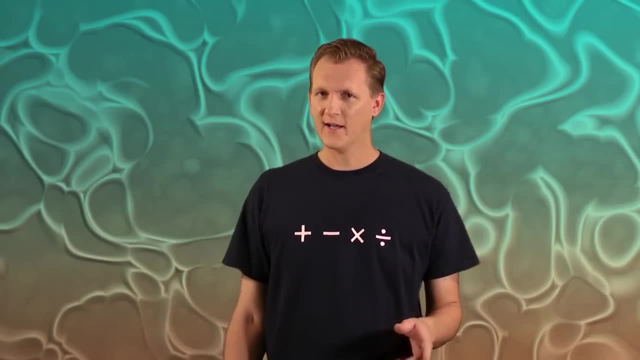 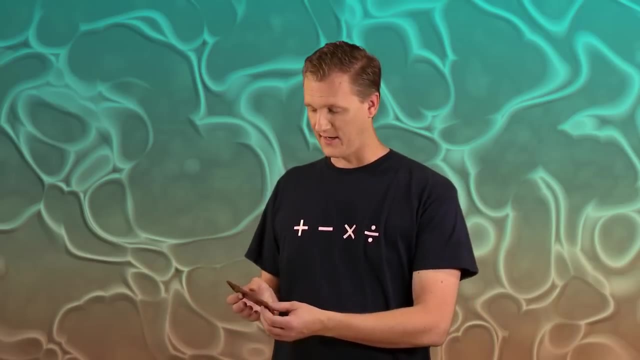 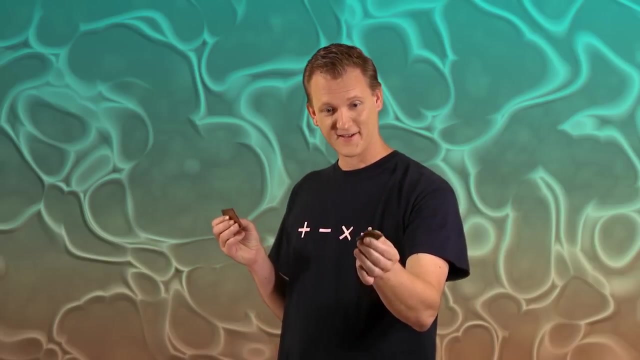 Oh, and it's important to remember that for fractions to work right, the parts that you divide the whole up into have to be equal. We can't like well, take a candy bar and say I'm going to divide it into two parts, so this is your half and here's my half. 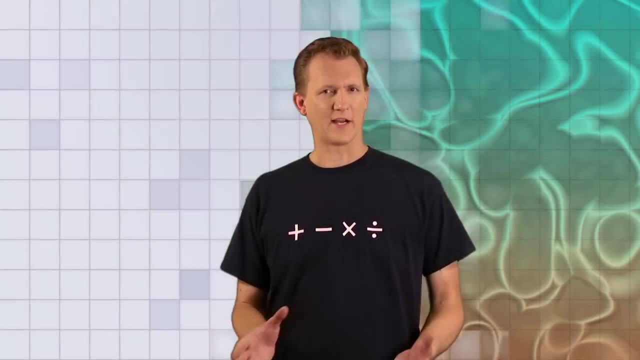 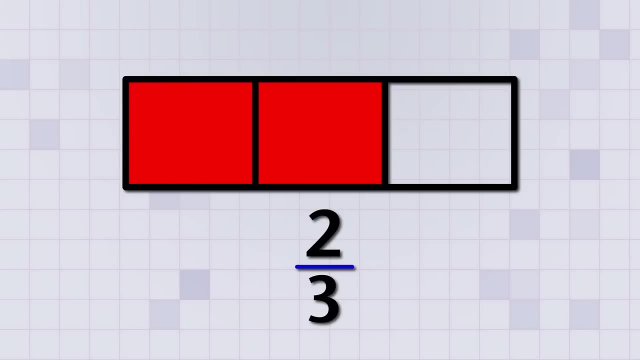 Let's look at a few more examples and really see the pattern of how fractions can represent parts of objects. This rectangle is divided up into three equal parts and two of them are shaded red. So two over three or two-thirds of the rectangle is shaded red. 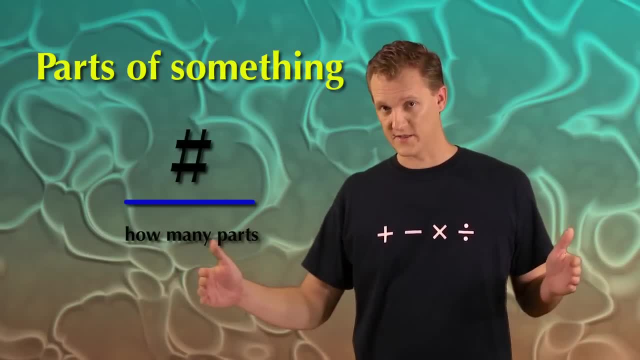 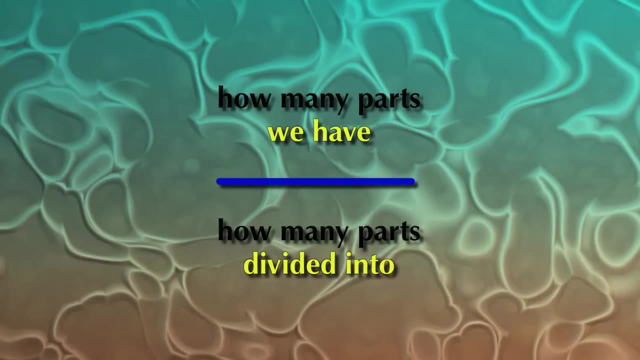 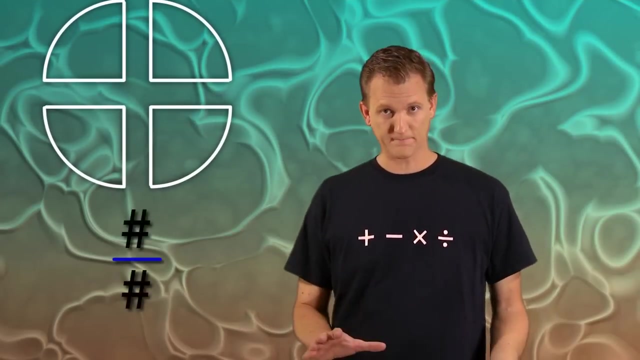 And the number on the bottom tells us how many parts that something is divided into. The number on top tells us how many of those parts we have. For example, let's write a fraction for our drawing here. I divided the circle into four parts, right? 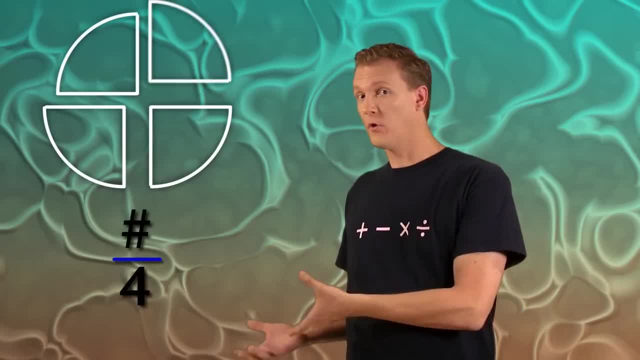 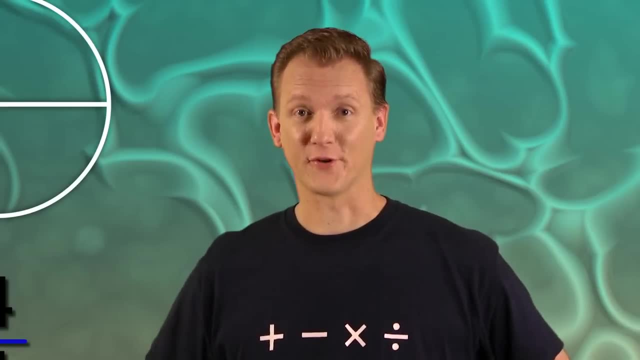 So the number on the bottom will be four. And I still have all four of those parts. so the number on top will also be four. I have four out of four parts. That means I still have a whole circle. But what if somebody came by and took away one part from the circle? 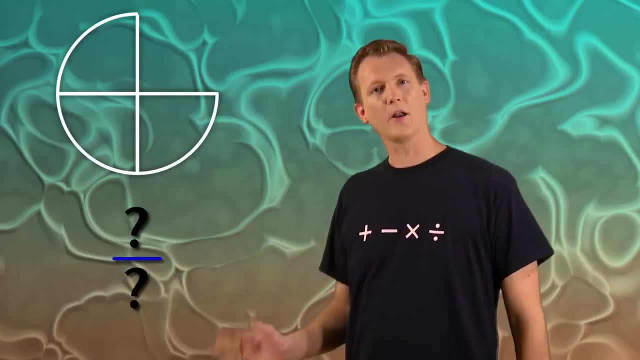 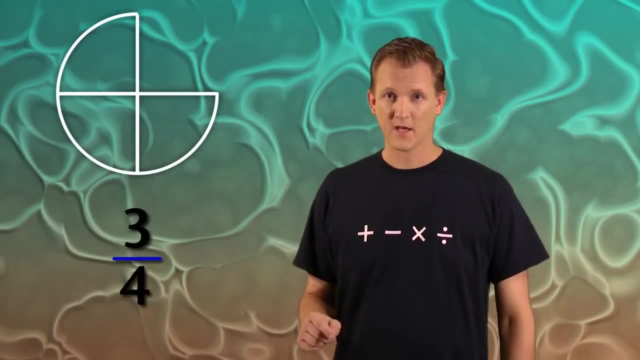 Well, the circle's still divided into four parts, so the bottom number would still be four. But I only have three of those parts left, So that means the top number will change to three. So I have three over four or three-fourths of a circle. 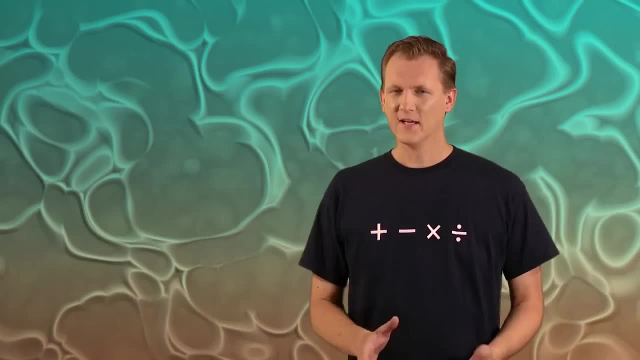 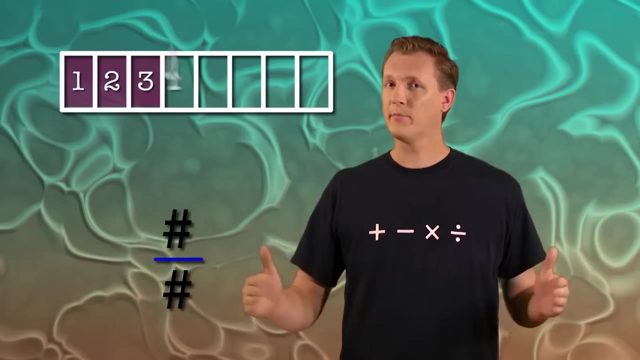 Make sense. so far Good. Let's try another example. Let's say that I divide a rectangle up into eight parts And I give you three of those parts. Since the total number of parts is eight, the bottom number will be eight. 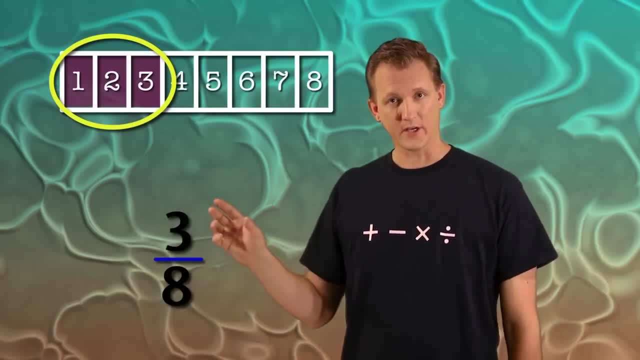 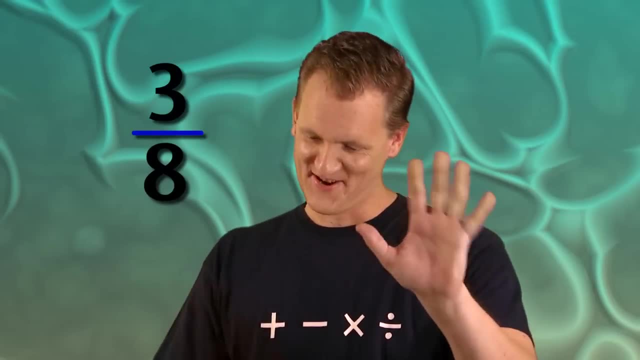 And since you have three of those parts, the top number will be three. So the fraction I'm giving you is four. That means three over eight or three-eighths of the rectangle. No, no, no, No need to think. 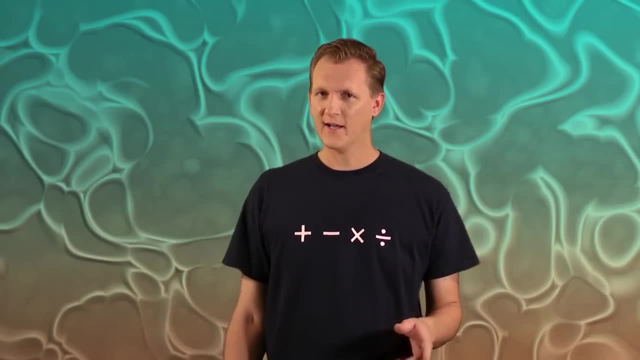 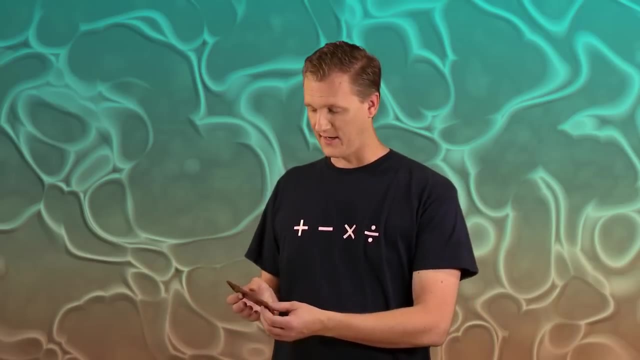 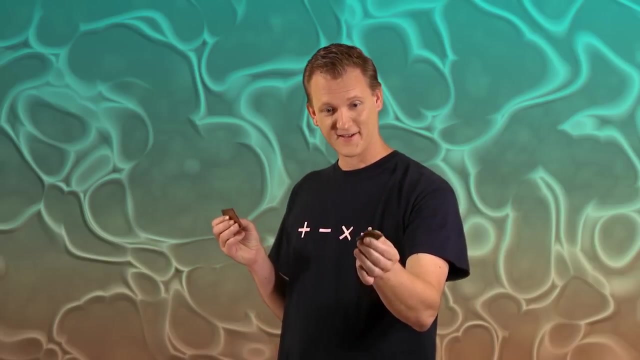 Oh, and it's important to remember that for fractions to work right, the parts that you divide the whole up into have to be equal. We can't like well, take a candy bar and say I'm going to divide it into two parts, so this is your half and here's my half. 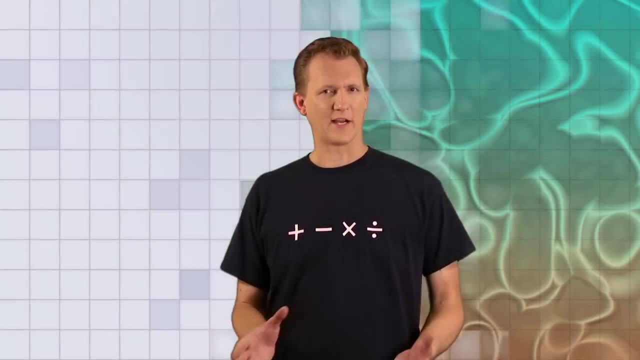 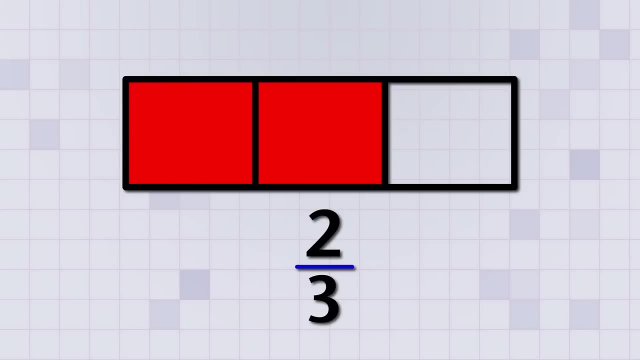 Let's look at a few more examples and really see the pattern of how fractions can represent parts of objects. This rectangle is divided up into three equal parts and two of them are shaded red. So two over three or two-thirds of the rectangle is shaded red. 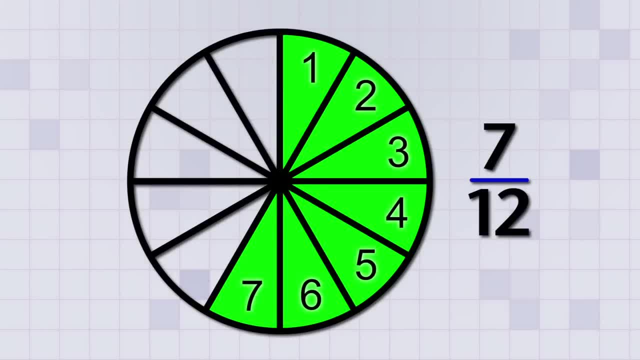 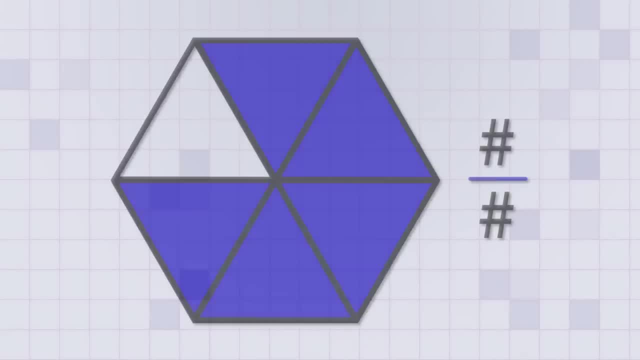 The circle is divided into twelve equal parts, and seven of those parts are shaded green. So seven over twelve or seven-twelfths of the circle is shaded green. The hexagon is divided into six equal parts, and five of those parts are shaded blue. 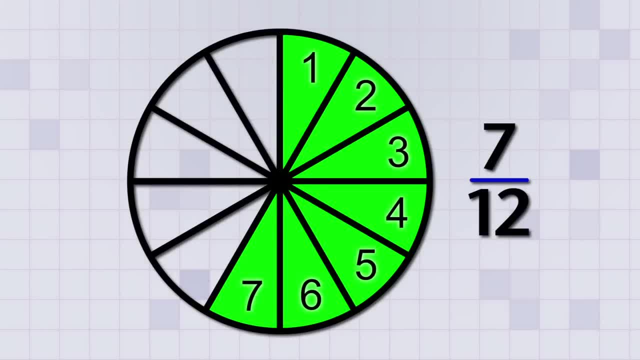 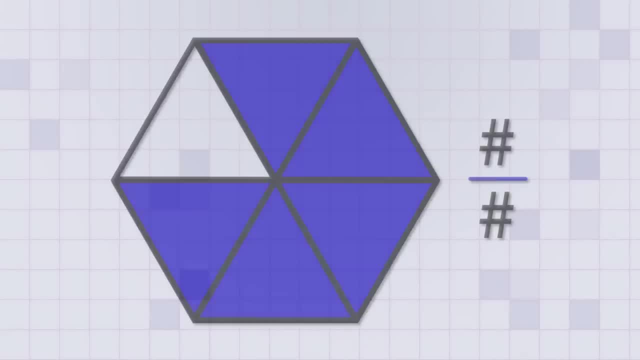 The circle is divided into twelve equal parts, and seven of those parts are shaded green. So seven over twelve or seven-twelfths of the circle is shaded green. The hexagon is divided into six equal parts, and five of those parts are shaded blue. 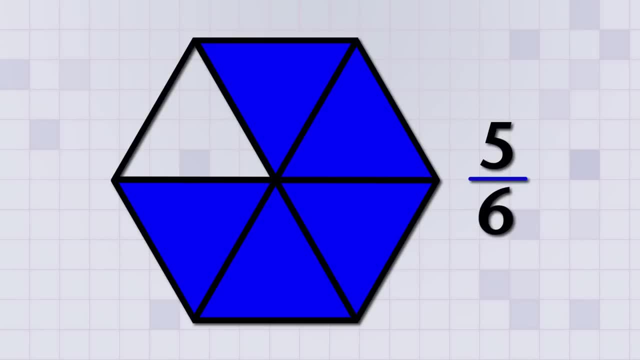 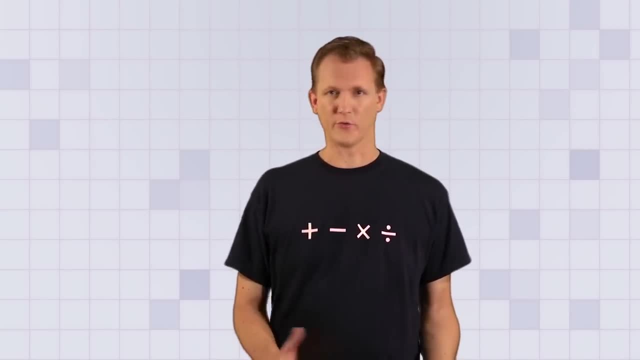 So five over six or five-sixths of the hexagon is shaded blue. Alright, so you can see how fractions can be used to represent parts of objects like circles and rectangles, But fractions can be used for more than that. They can be used to represent parts of well anything. 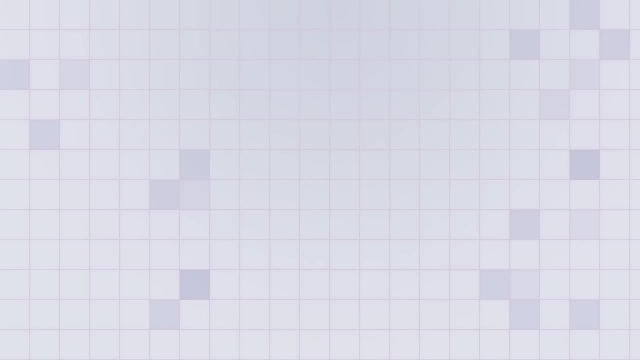 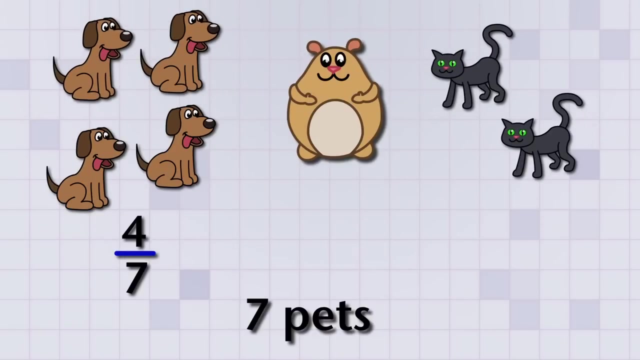 Like like pets. for example, Let's say you have seven pets: Four dogs, two cats and a big fat hamster. Well, that means that four over seven or four-sevenths of your pets are dogs. 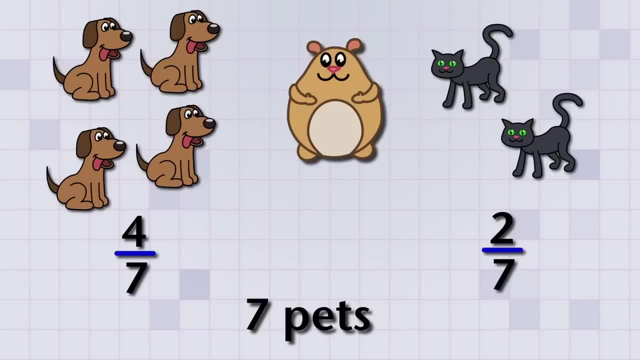 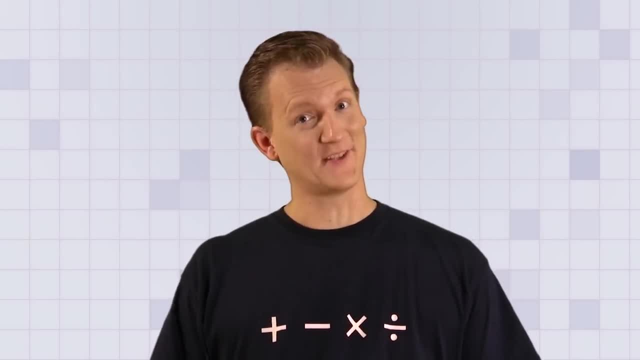 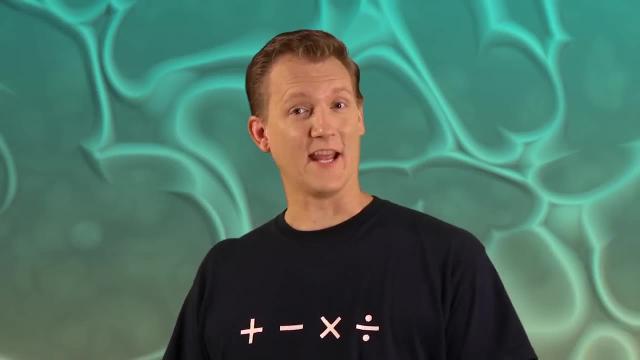 And two over seven or two-sevenths of your pets are cats And one over seven or one-seventh of your pets are hamsters. It also means that your house probably smells like a pet store. Okay, So fractions can be used to represent anything from parts of a circle to kitty cats. 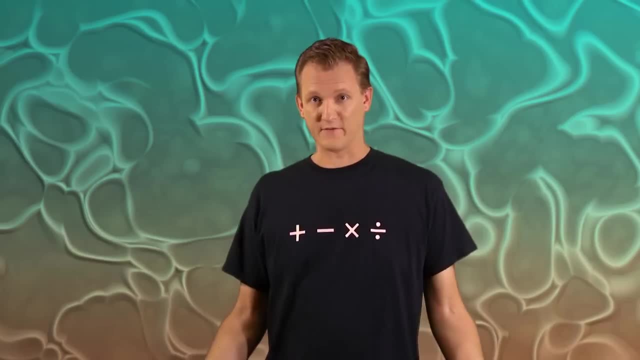 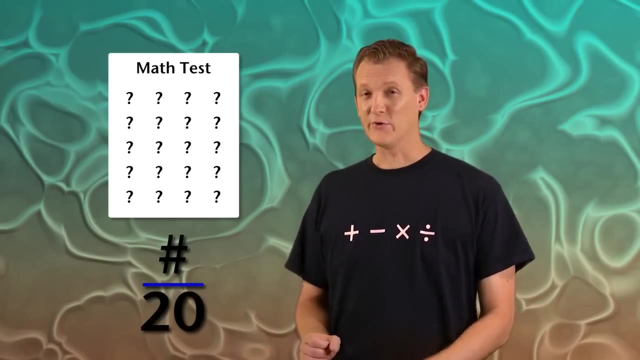 But did you know that fractions can also be used to represent things you can't even see Well, like a test score, for example? Let's say you take a math test and there's twenty questions on the test, And you get seventeen of those questions right. 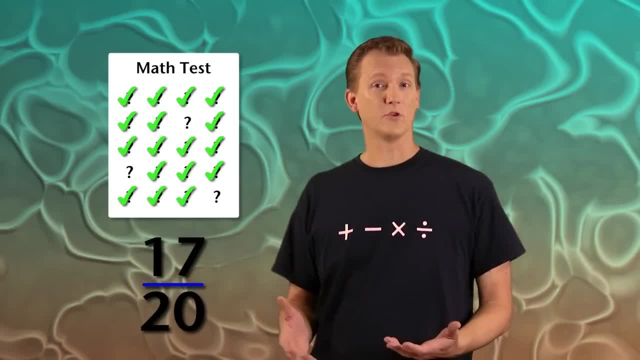 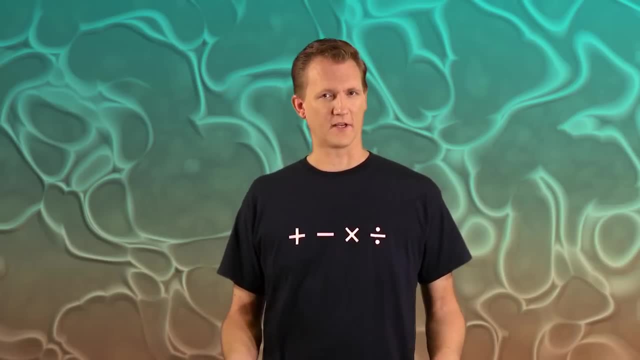 That means that you got seventeen, over twenty or seventeen-twentieths of the questions right, Alright. So that's the basic idea of how fractions can be used to represent parts of things, But there's a lot more to fractions than that. 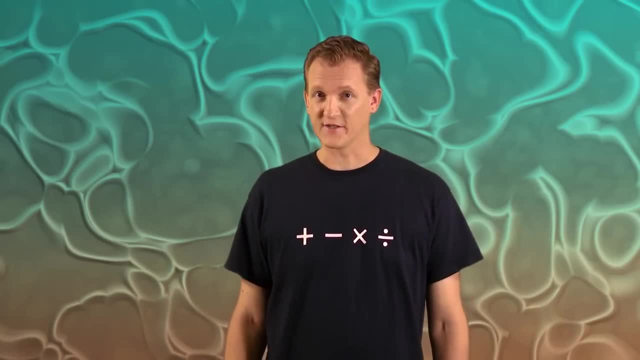 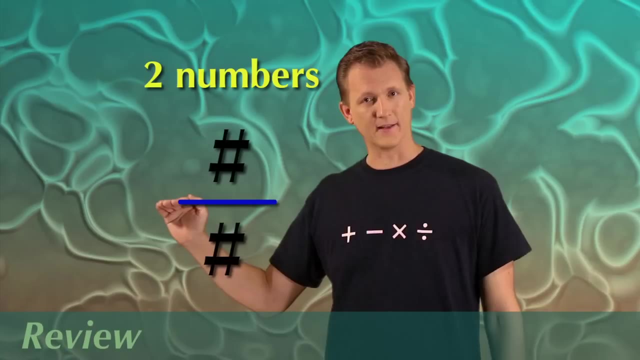 In the next section we're going to be looking at some of the other things we can do with fractions, But before that let's review. Fractions are used to represent parts of a whole. Fractions are written in the form of a top number over a bottom number, with a line between them. 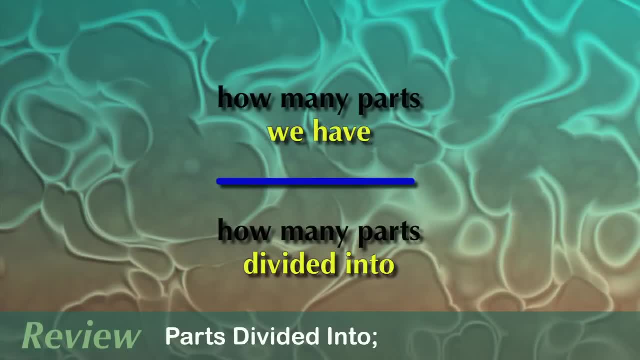 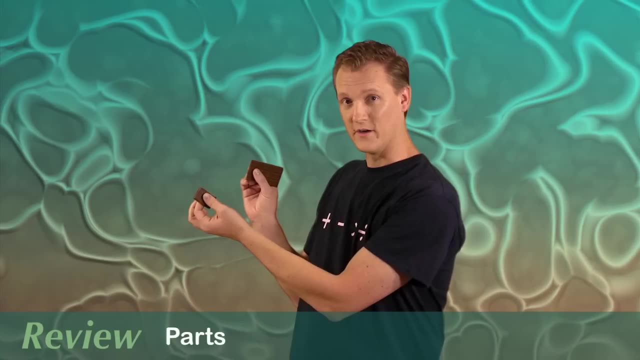 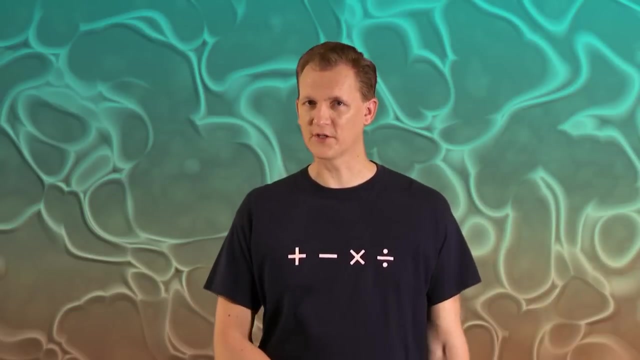 The bottom number represents how many parts the whole is divided into And the top number represents how many of those parts you have. And finally, the parts that a whole is divided up into must be equal for fractions to work right. To really understand how fractions are used to represent parts of things, be sure to do the exercises. 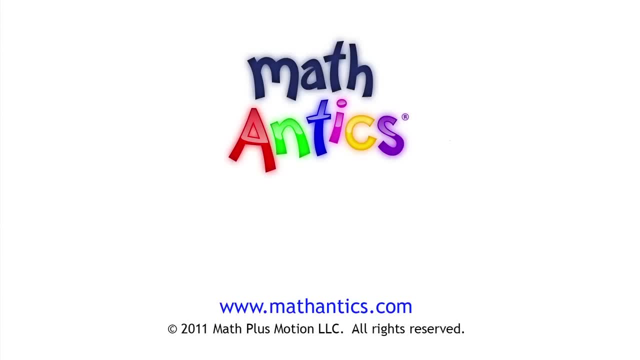 And I'll see you in section two. Learn more at wwwmathanticscom. 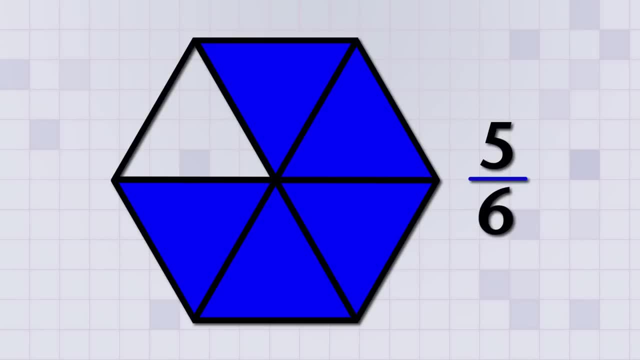 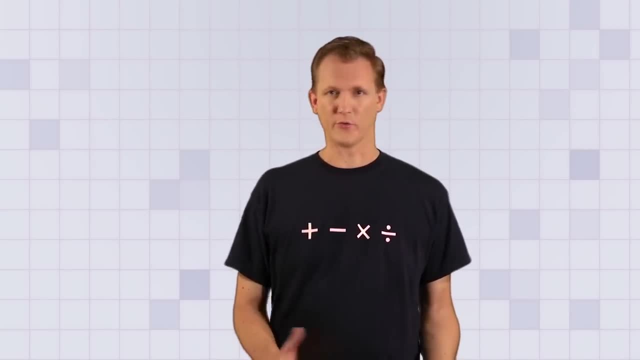 So five over six or five-sixths of the hexagon is shaded blue. Alright, so you can see how fractions can be used to represent parts of objects like circles and rectangles, But fractions can be used for more than that. They can be used to represent parts of well anything. 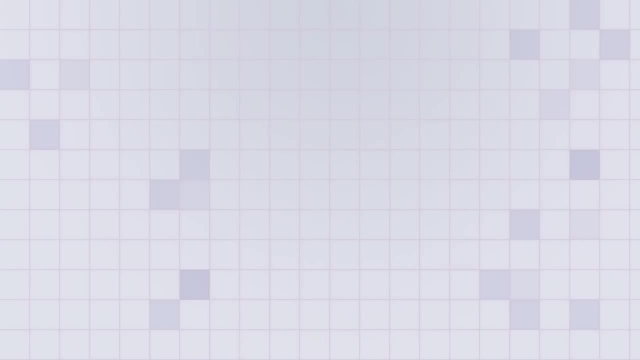 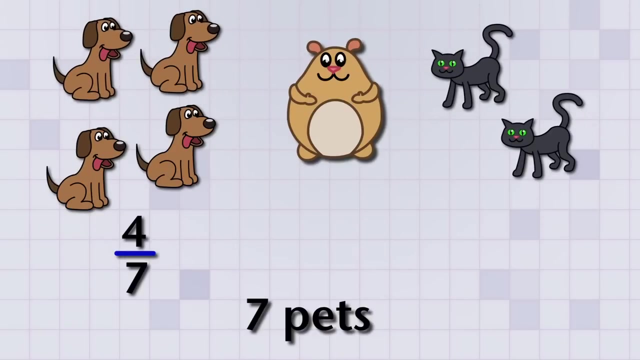 Like like pets. for example, Let's say you have seven pets: Four dogs, two cats and a big fat hamster. Well, that means that four over seven or four-sevenths of your pets are dogs And two over seven or two-sevenths of your pets are cats. 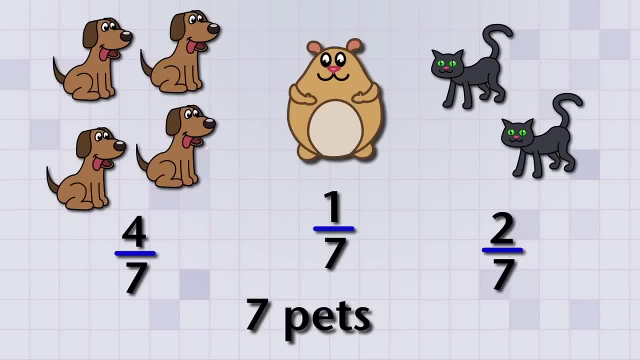 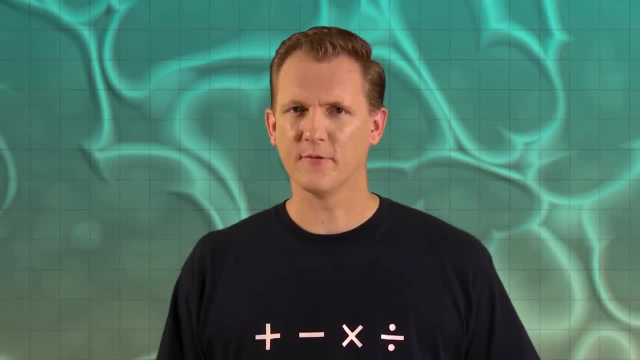 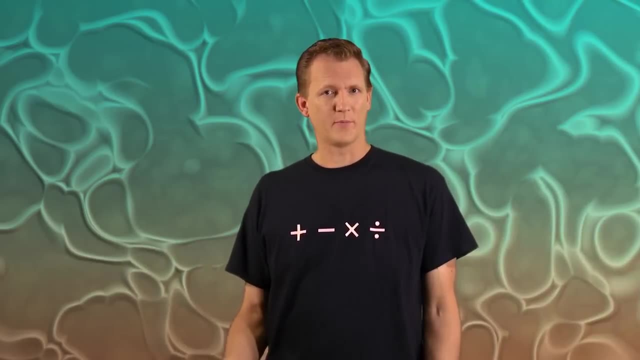 And one over seven or one-seventh of your pets are hamsters, It also means that your house probably smells like a pet store. Okay, So fractions can be used to represent anything from parts of a circle to kitty cats, But did you know that fractions can also be used to represent things you can't even see? 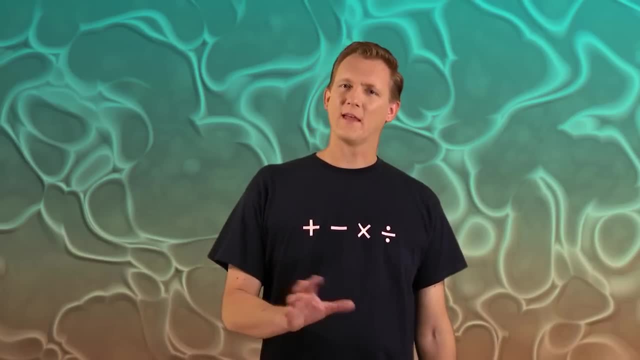 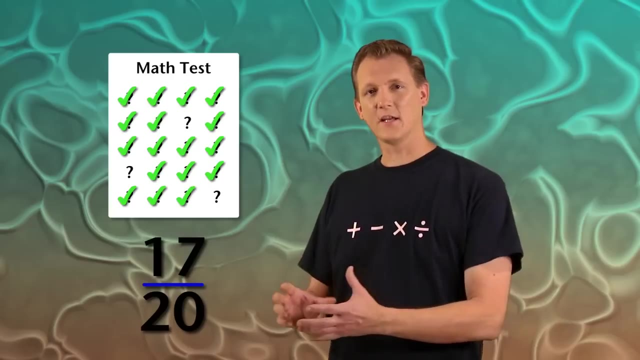 Well, like a test score. for example, Let's say you take a math test and there's twenty questions on the test And you get seventeen of those questions right. That means that you got seventeen over twenty or seventeen-twentieths of the questions right. 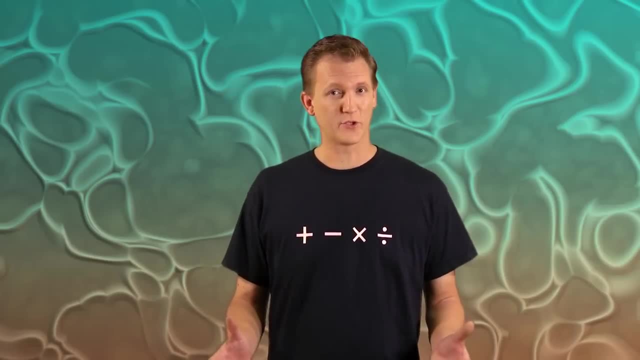 Alright. So that's the basic idea of how fractions can be used to represent parts of things, But there's a lot more to fractions than that. In the next section, we're going to be looking at some of the other things we can do with fractions. 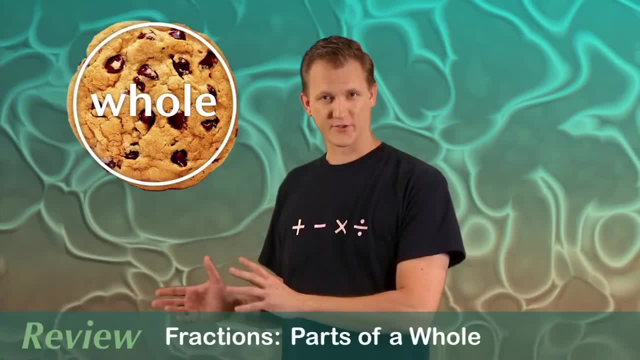 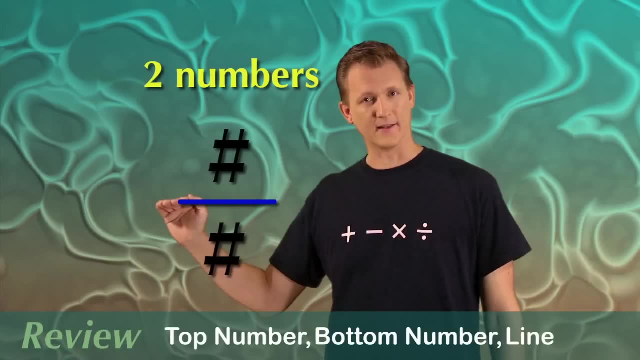 But before that let's review. Fractions are used to represent parts of a whole. Fractions are written in the form of a top number over a bottom number with a line between them. The bottom number represents how many parts the whole is divided into. 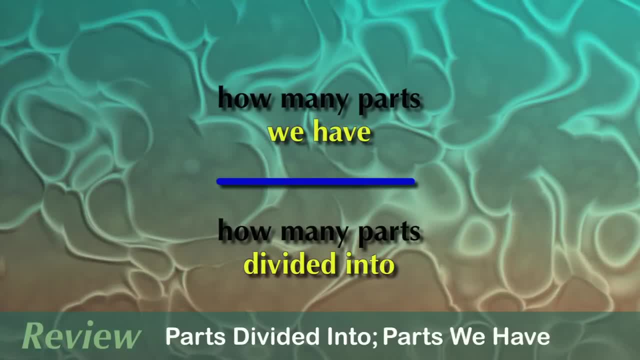 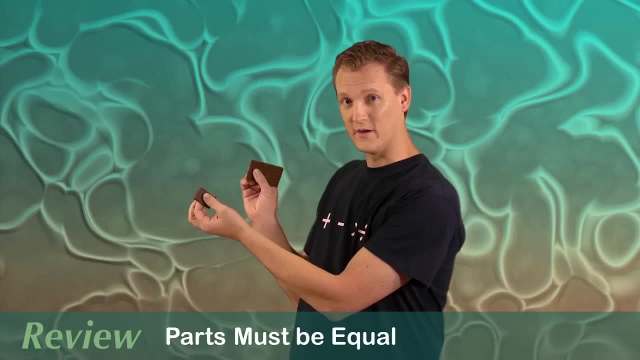 And the top number represents how many of those parts you have. And finally, the parts that a whole is divided up into must be equal for fractions to work right. To really understand how fractions are used to represent parts of things, be sure to do the exercises. 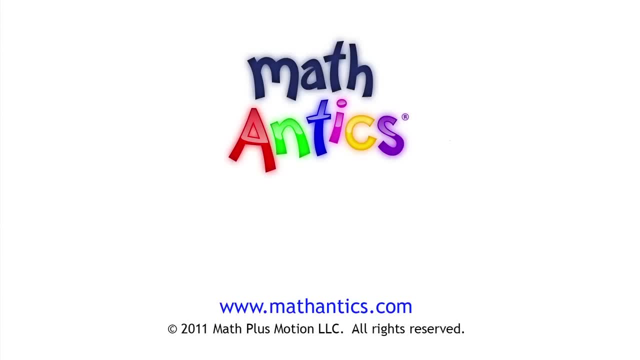 And I'll see you in section two. Learn more at wwwmathanticscom.